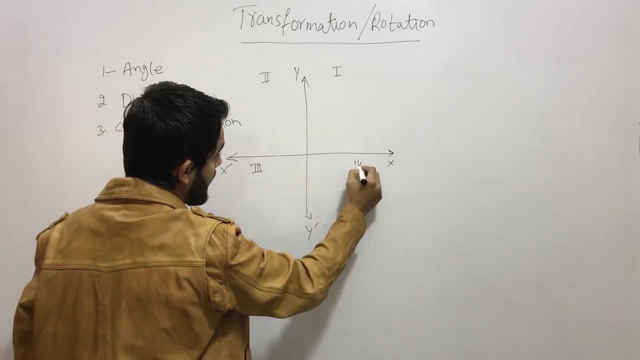 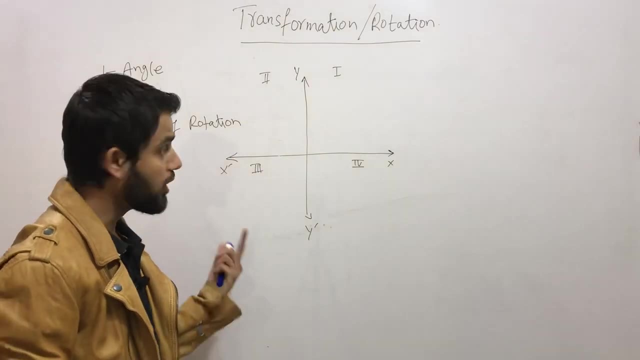 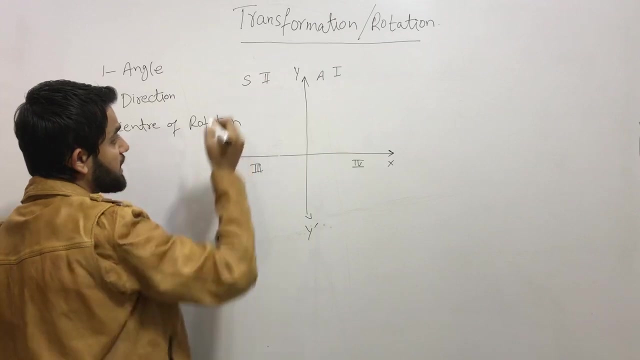 This is your second quadrant, and here is your third quadrant, And over here we have our fourth quadrant. On these four quadrant, we always know that over here, all positive, We can say all positive. Over here only sine is positive. Over here only tan is positive. 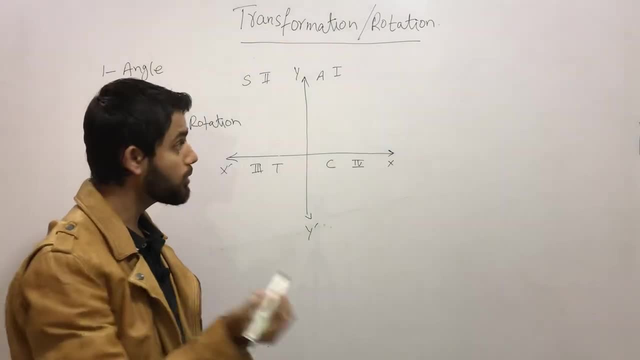 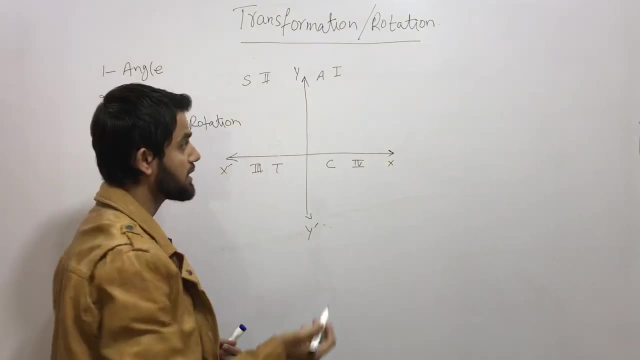 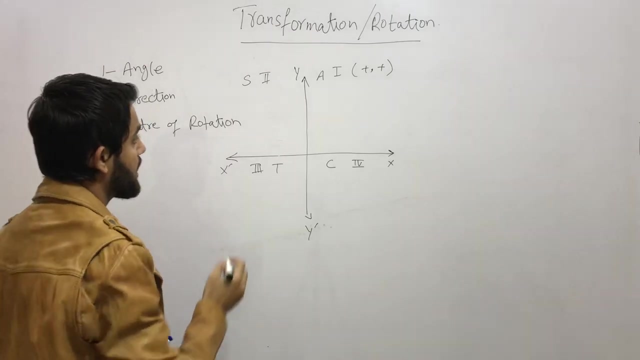 And over here only cos is positive. What do I mean by that? On x axis we always take cos theta axis we always take sine theta. so when all are positive, it means that x axis is positive, y axis is positive. over here, in this quadrant, over here we have only sine is positive. it means that x is. 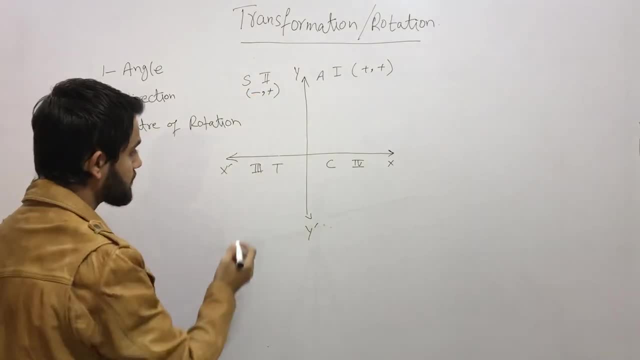 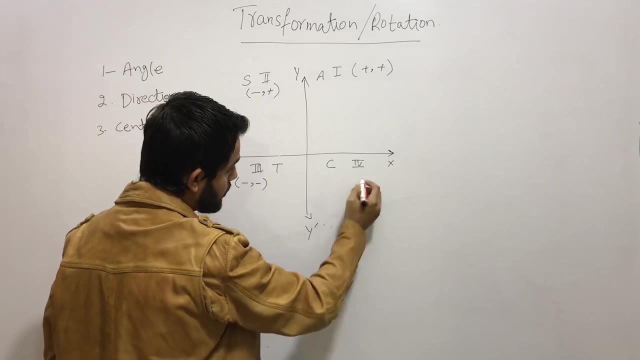 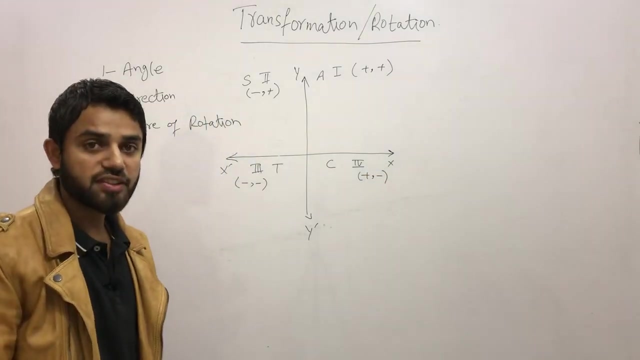 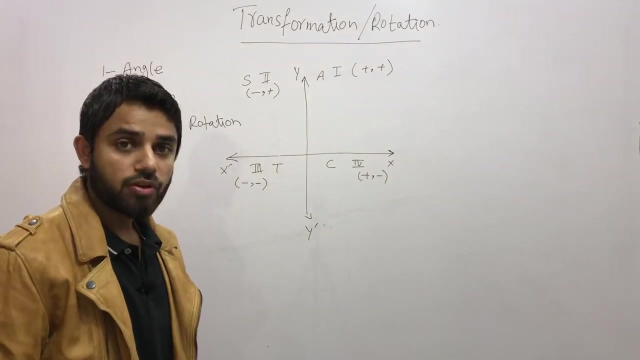 negative and y is positive. over here on this plane, both are negative on this. on this quadrant- fourth quadrant- we have only cos positive, so means that x is positive and y is basically negative. so this is the basic about x- y plane. okay, so what i am going to do now? i am going to take a random figure. 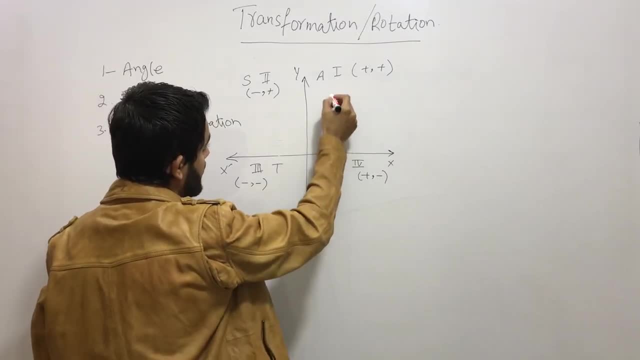 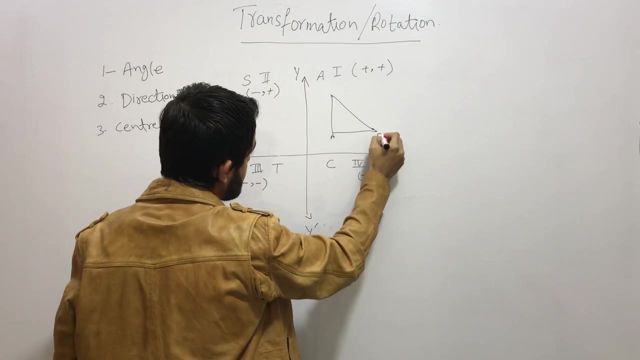 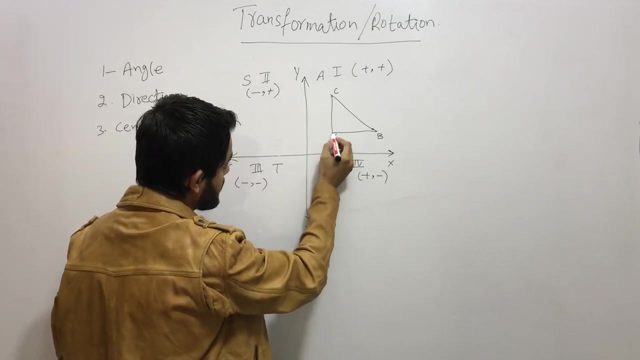 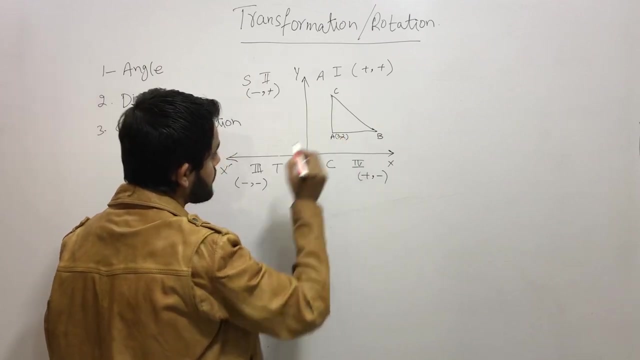 a right angle triangle over here. let's assume that this is the right angle triangle i am taking and the coordinates are a, b and c. the vertices are the eins Forum y axis. let's say that comm вн架 will be exactly the same on ead for Claro, which is basically same point. 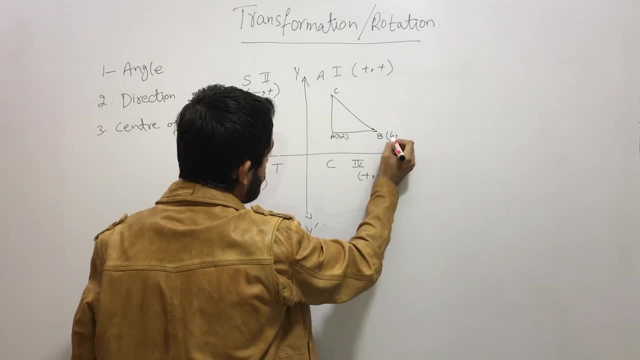 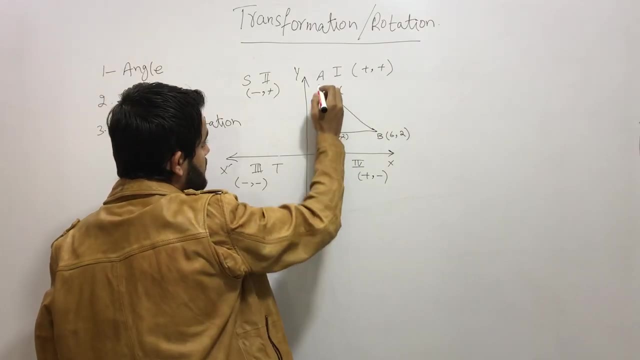 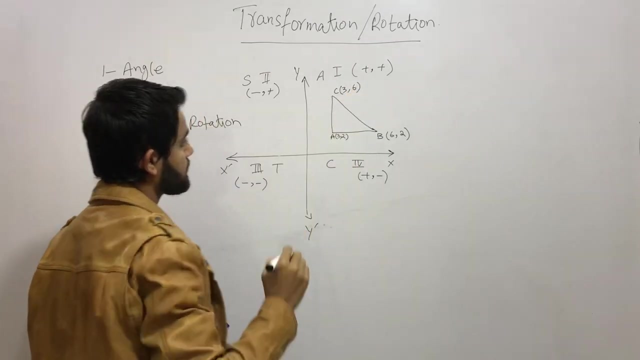 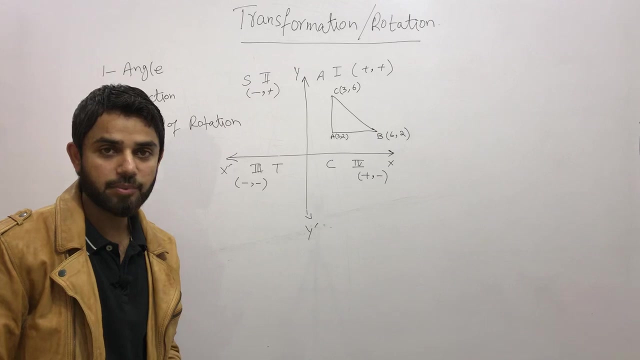 40 degree and e. so that's why we use�, we use between one on both, and it looks like the same just with different little details, and we are going to combine with each other. so let's say it is six on y axis. let's say it's six. so these are the three coordinate of a triangle: a, b, c. 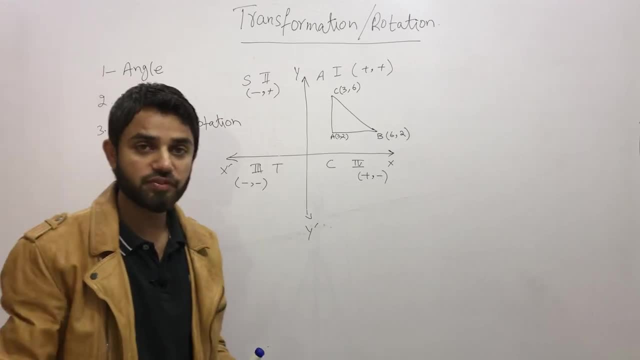 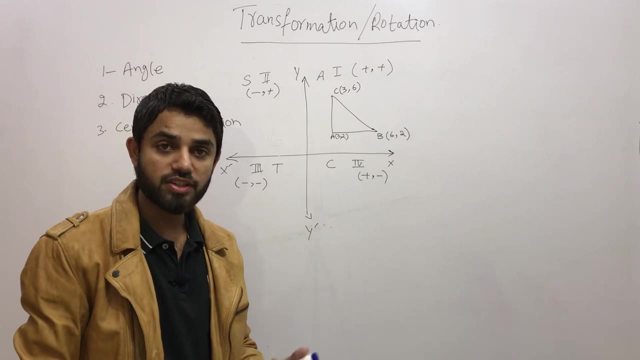 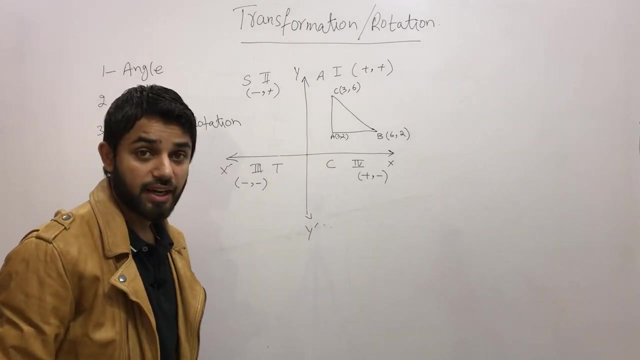 now what i am going to do now, what we will learn by the end of this video. we are going to learn the rotation on clockwise and we are going to learn the rotation and on anticlockwise as well, where we are keeping the center of rotation as center. at first, i am going to rotate this triangle. 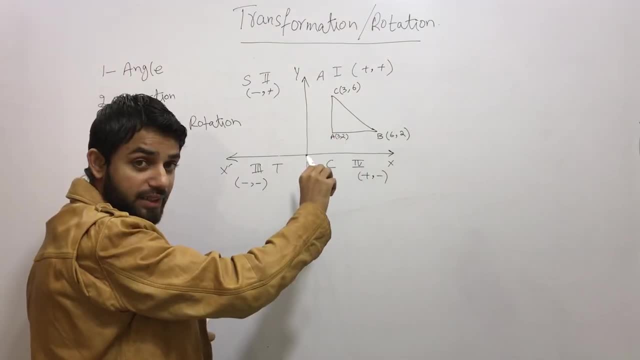 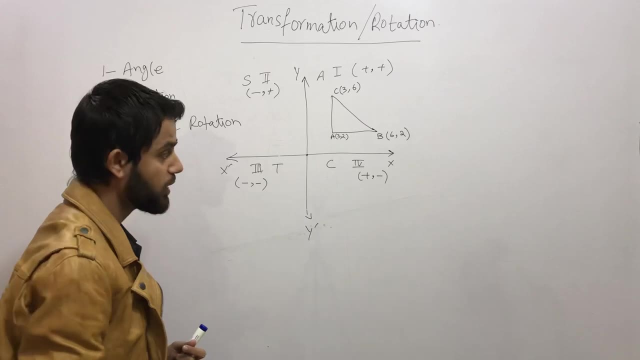 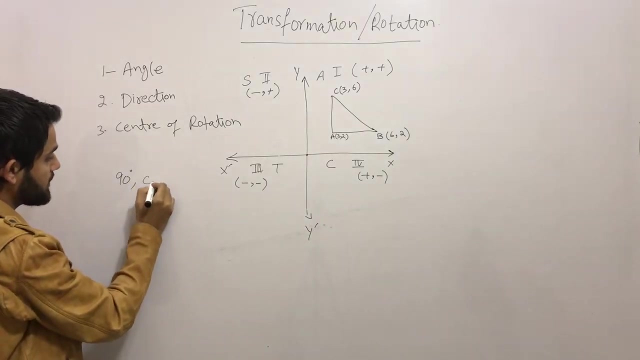 x, y, z on 90 degree along 90 degree by keeping this center of point on clockwise direction. so at first, 90 degree is the angle, the direction is basically clockwise. c dot w means that it's not actually a class work. it means that it's. 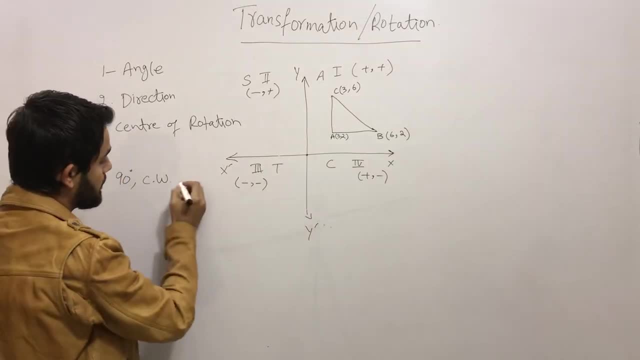 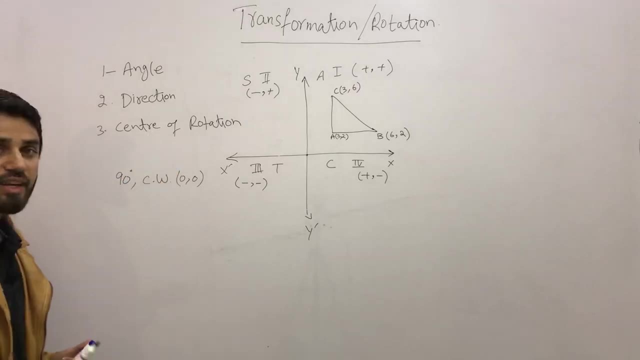 a clockwise. and the third, it means that center o comma o zero, comma zero. so i told you earlier, only these are the three things that we needed in order to rotate any figure or any object. this is your angle, this is the direction and this is the center of point where we want to rotate. 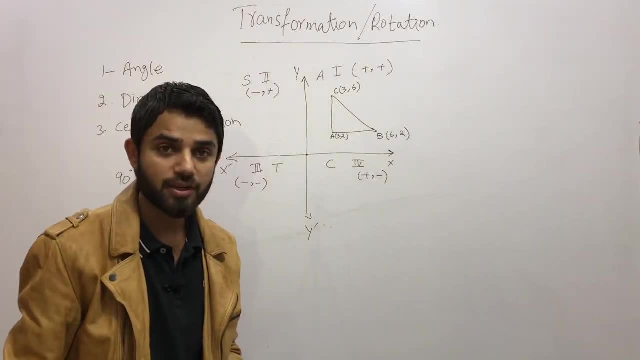 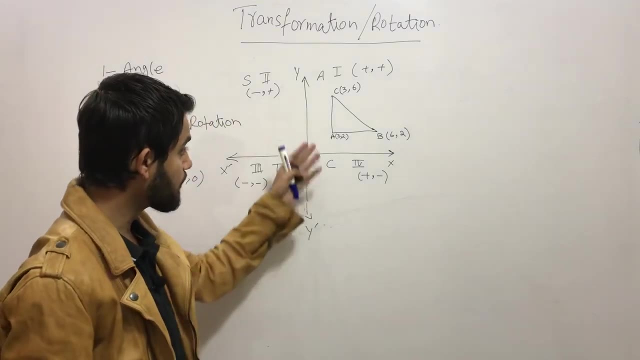 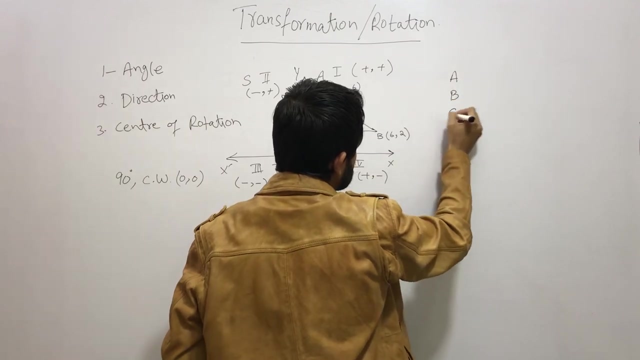 so in general, the student are doing the tracing method, but i i don't really like that tracing method. so what i'm going to tell you now? i'm going to give you another method in which you can rotate and figure very quickly and very easy. so let's write the point a, b, c over here, the. 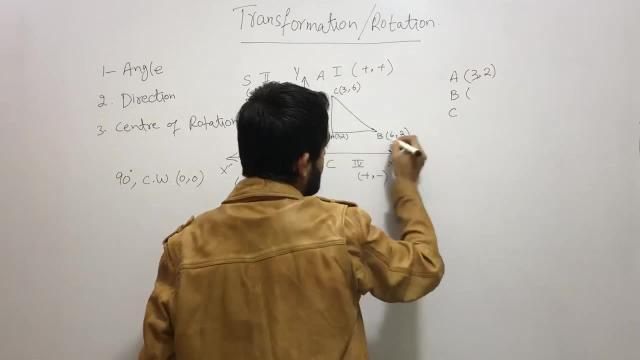 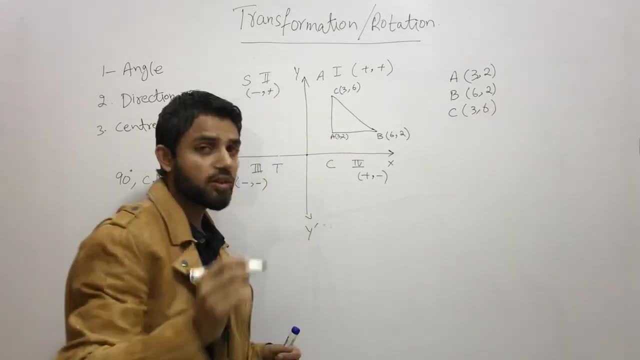 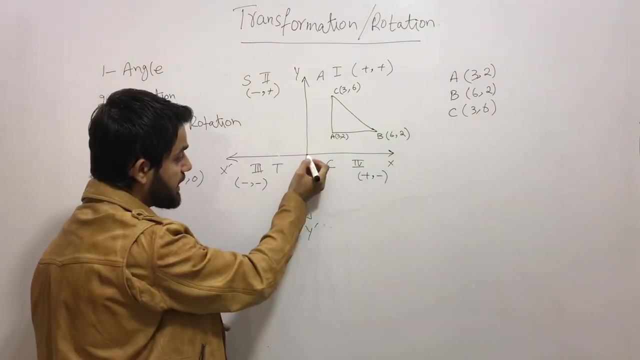 coordinates of a- r 3 comma 2, the coordinates of b- r 6 comma 2, and the coordinate of c- r 3 comma 6, once you are rotating an object in clockwise direction by keeping your center as origin, what you need to do so? 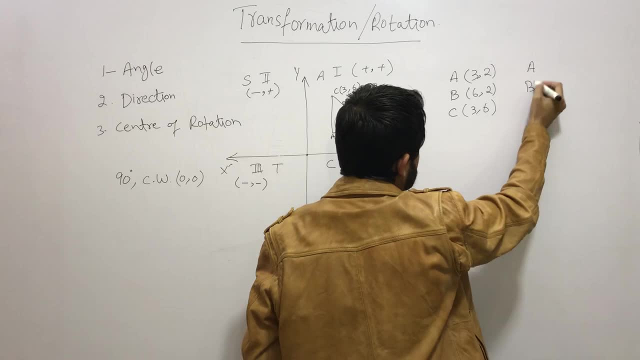 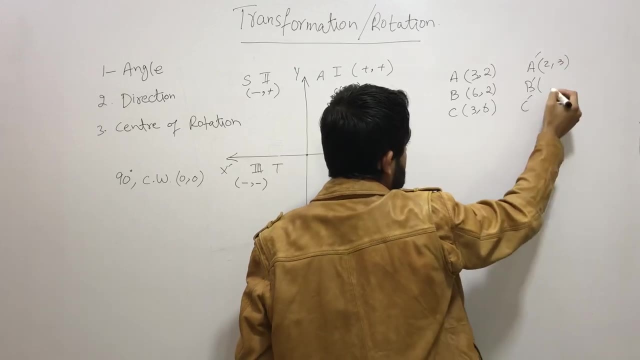 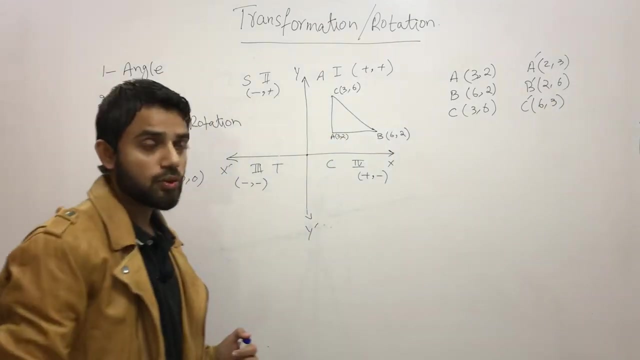 simply switch the places. what do i mean by that? it take it as 2- 3, take this as 2 comma 6 and take this as 6 comma 3. now you need to know your original position. our original position is on the first quarter. 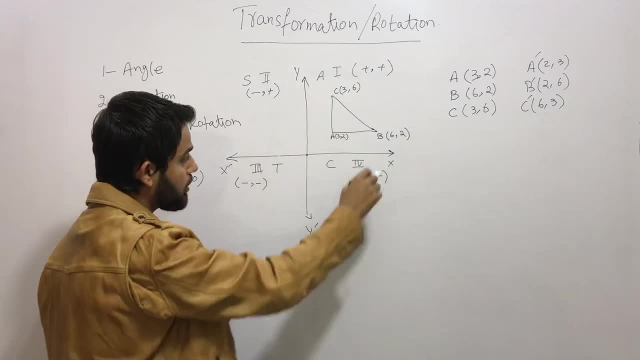 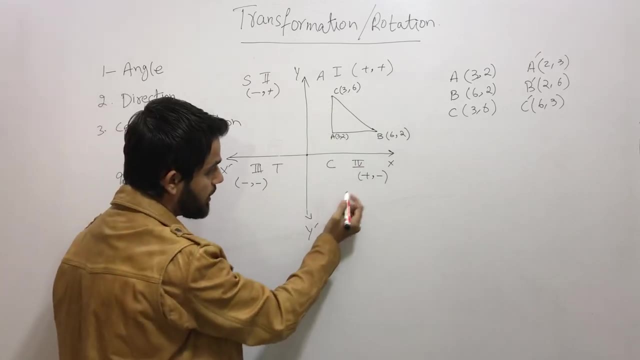 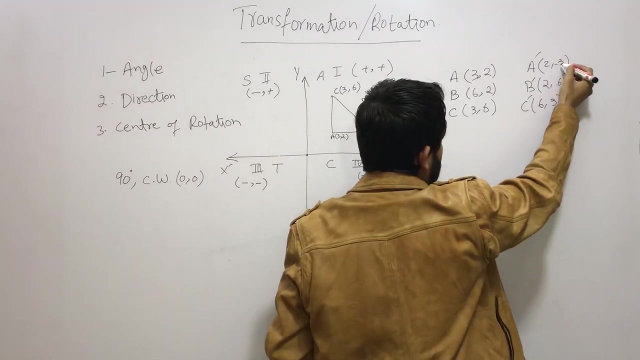 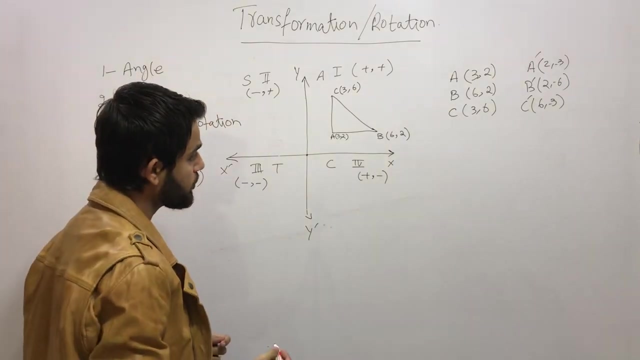 and we are rotating it clockwise. so once we are rotating it clockwise, it means that from the first quadrant we are coming into the fourth quadrant. now, in this fourth quadrant, x suspend your positive and y axis is your negative. so, body, write the minus sign over here in all these 3. now draw these points. the first point a is 2 comma minus 3 and x. 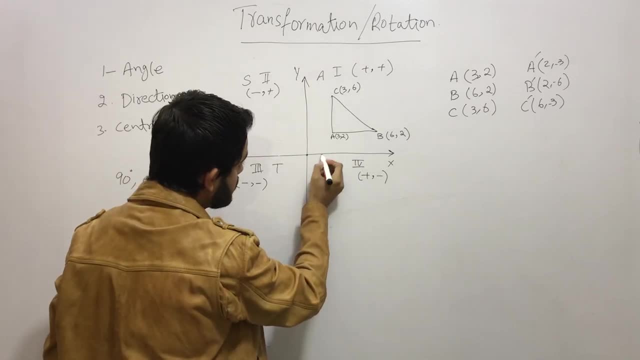 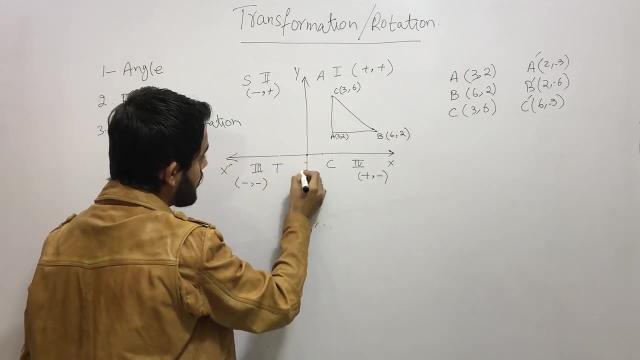 axis is 2, so over here it was 3, so 2 will be slightly behind, and y axis minus 3. so here you go: minus 1 minus 2. minus 1 that's equal to probability rate, which means that it is negative. i will be dividing the basis, so if i reduce from here like this negative sign: 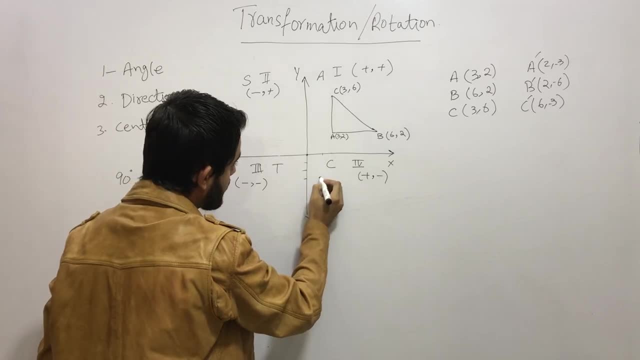 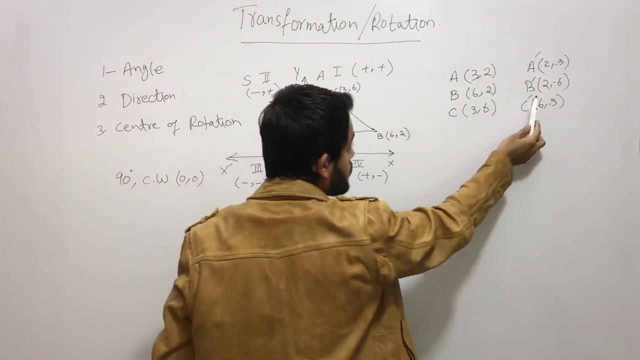 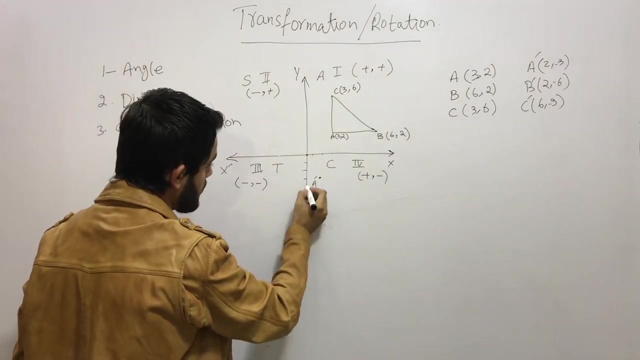 Minus 2 and minus 3.. So this is the first point that we have got a Prime which is minus 2 comma minus 3. now the second point B is 2 comma Minus 6.. So this is our 2, 1, 2 minus 6, 3, 4. 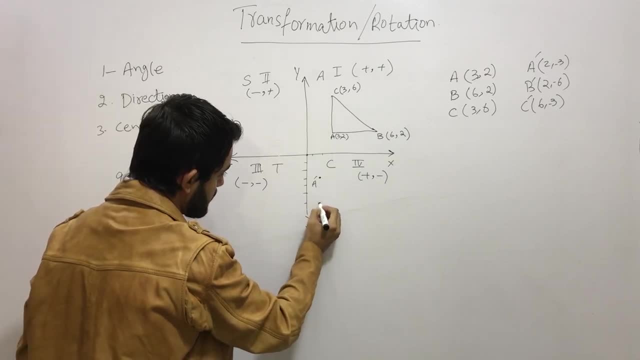 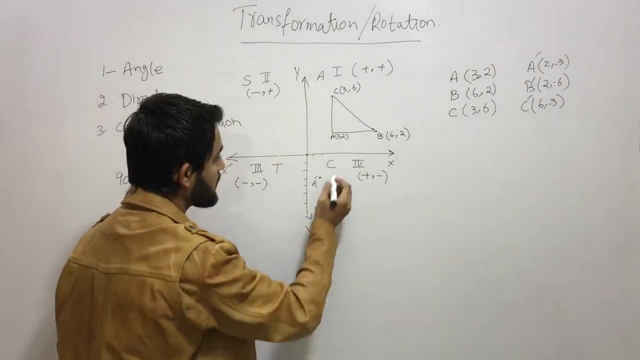 5 and 6, so 2 comma minus 6. This is our B prime, and C prime is 6 comma minus 3. on x-axis It's 6, So 6 we have here and minus 3, 1, 2, 3. 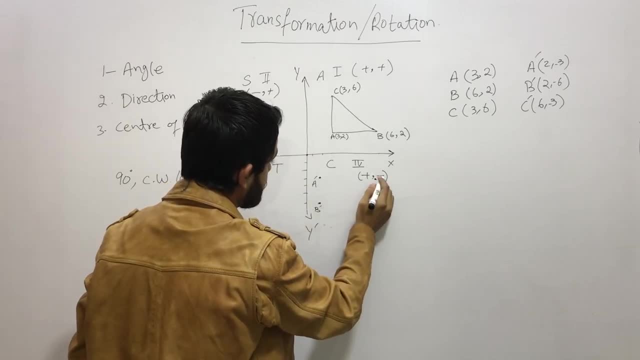 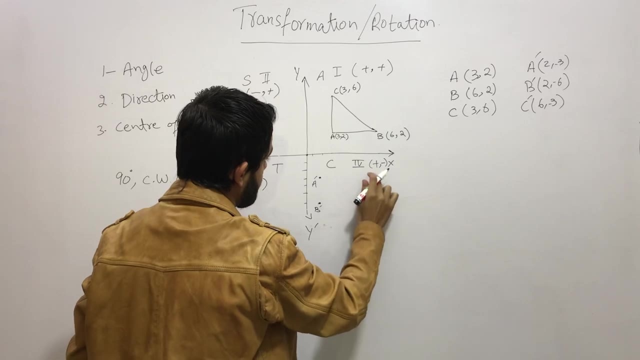 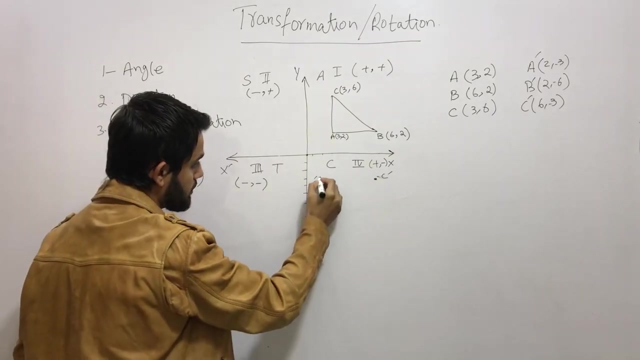 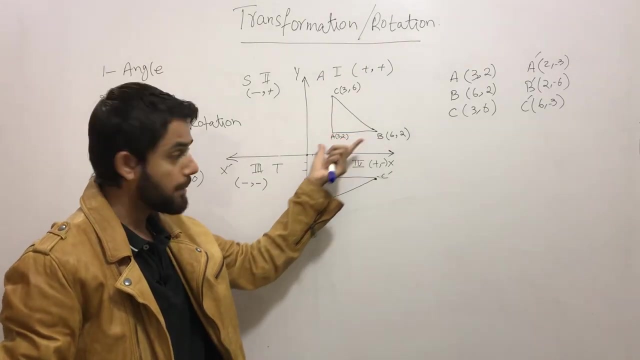 So we will be coming over here. So this is going to be- I should write it over here- plus minus. okay, so this is the point that we have got as C prime. now join these three point Together and you see we have rotated our triangle by. 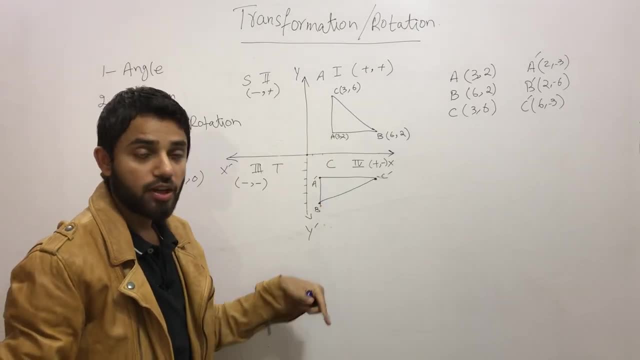 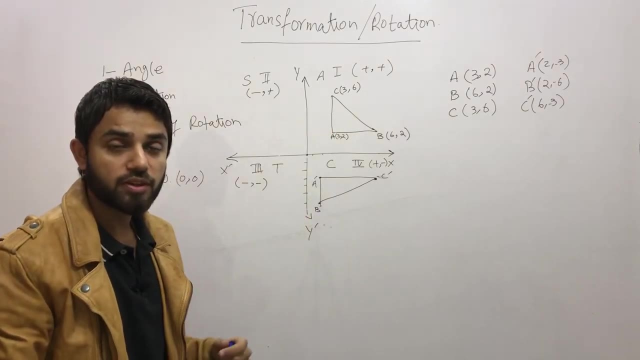 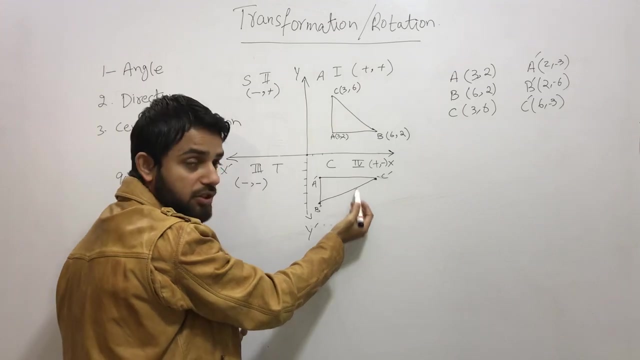 Keeping this center 90 degree clockwise. So what if? if I am moving now? one more thing that I would really like to highlight over here: Why we are moving to the anti-clockwise direction. This is your Object and this is your image. The original figure is basically going to called as object and this is going to be your image. now. 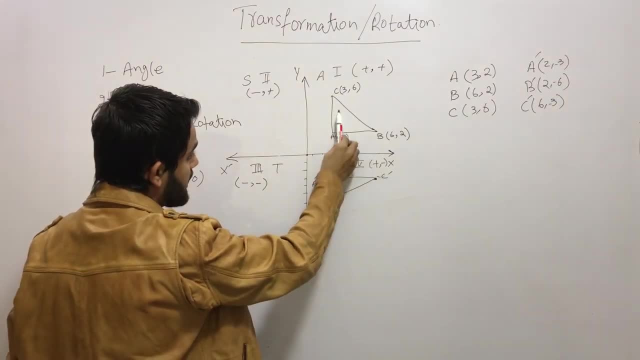 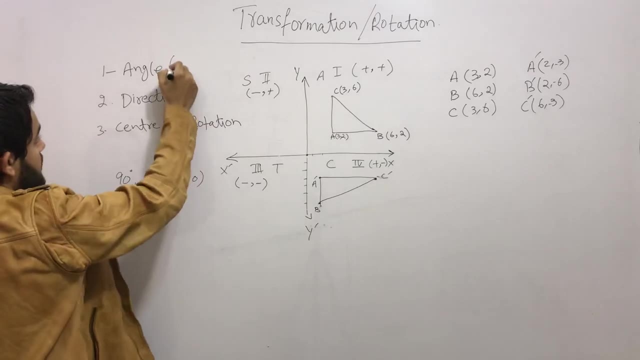 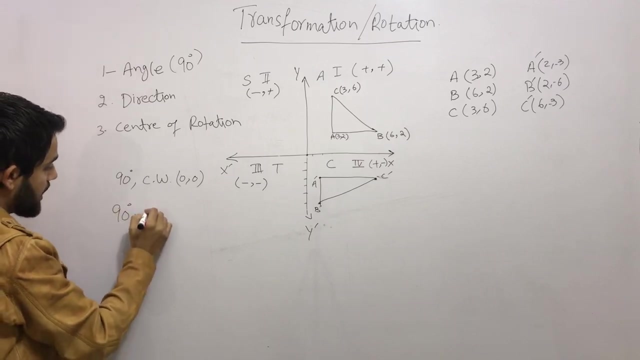 I want to move the same triangle ABC that we have over here into anti-clockwise Direction, 90 degree. So I am keeping the angle, 90 degree. Now the direction initially I took clockwise, so 90 degree, Anti-clockwise direction, and the center of point I am going to take is basically 0 comma 0. 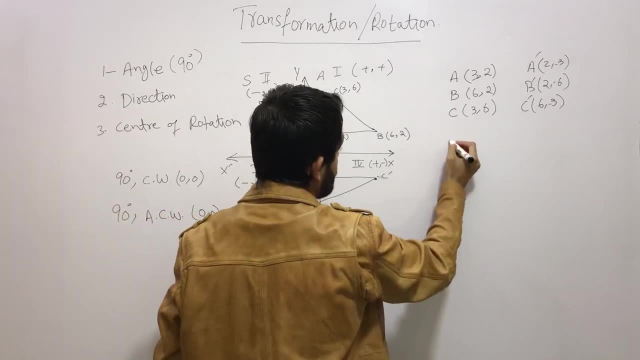 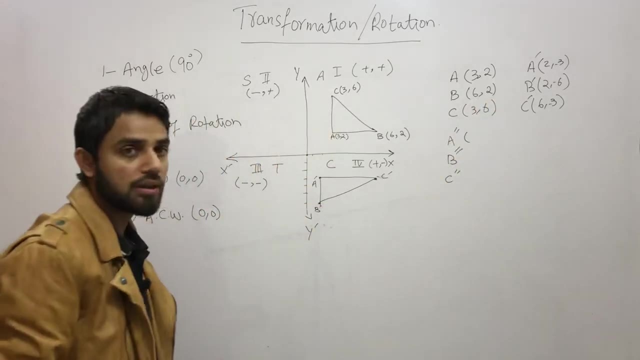 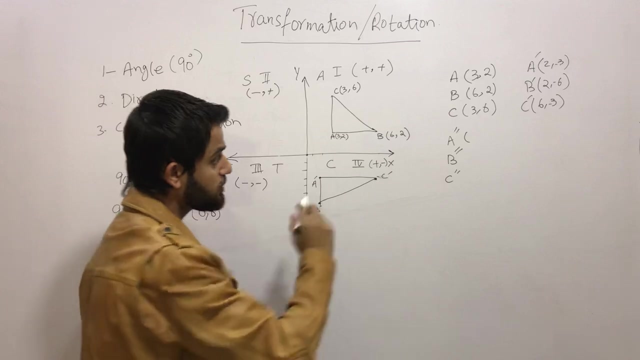 So again we will be using the same formula. So a prime, B prime and let's say double prime, So to keep it, the difference between all these three point. So every time when you're rotating an object 90 degree. so what do you need to do? just switch the point X, comma Y. 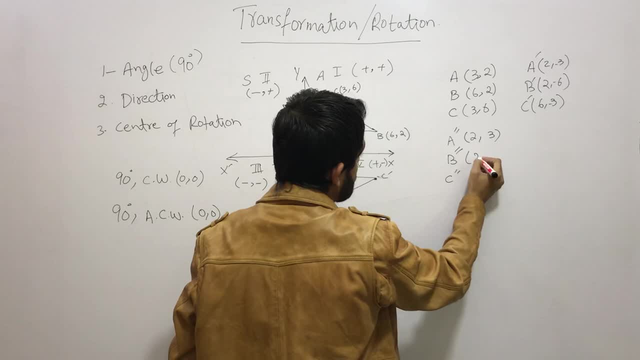 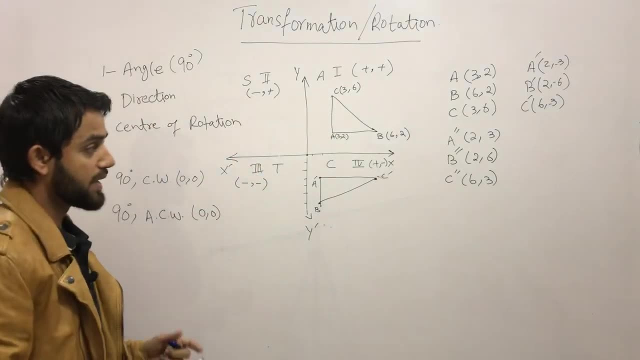 so it's going to become 2 comma 3, this is going to become 2 comma 6, and this was 3 comma 6. it will be 6 comma 3. Now again. now you need to identify your original position, where you are having your figure. 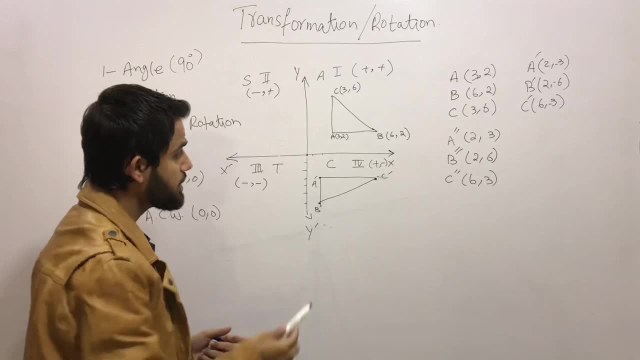 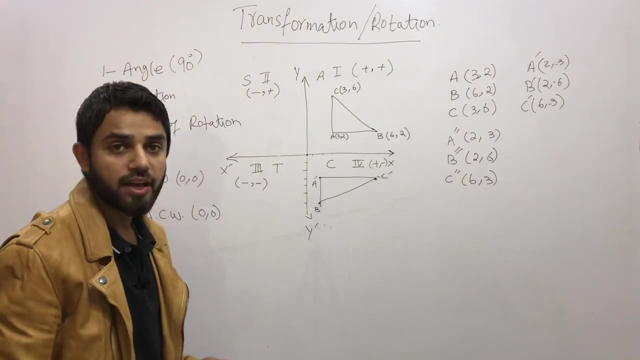 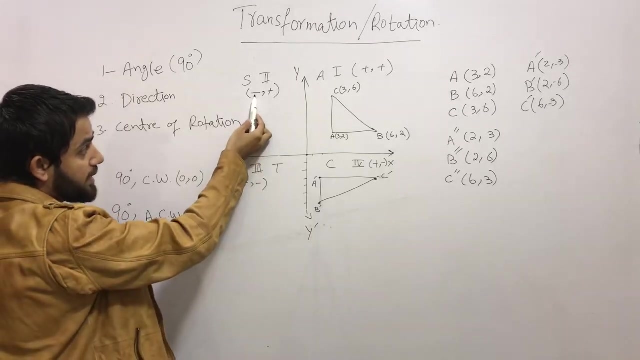 The original position is on the first quarter. now, once I'm shifting it to the anti-clockwise direction, 90 degree, it means that i will end up over here in the second quadrant. now, in this second quadrant, your x is negative and y is positive. so write negative values for all the x-axis. so this is. 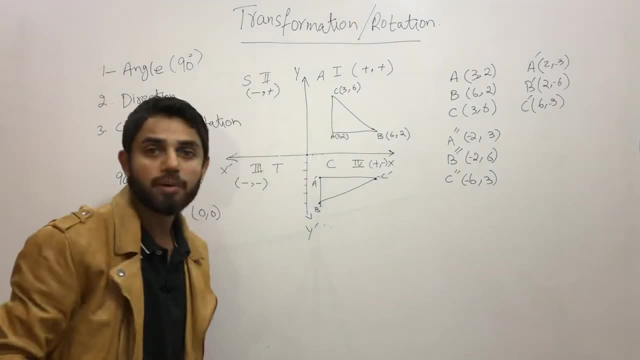 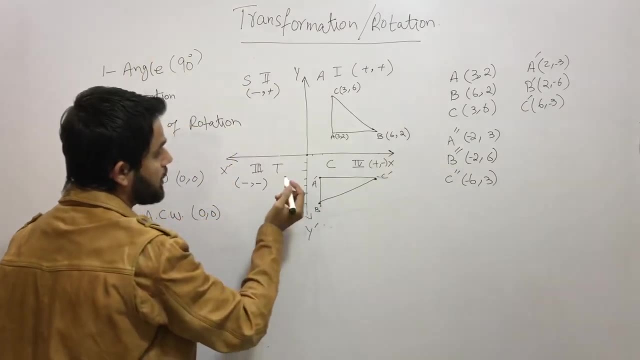 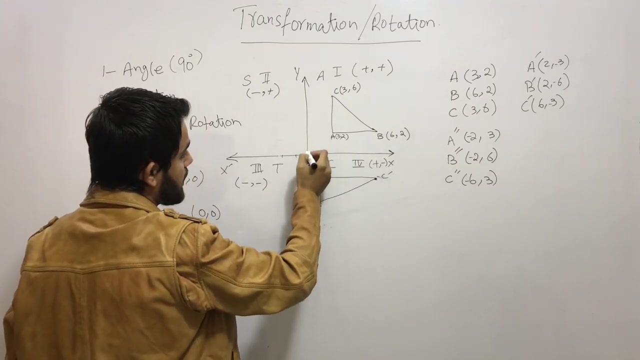 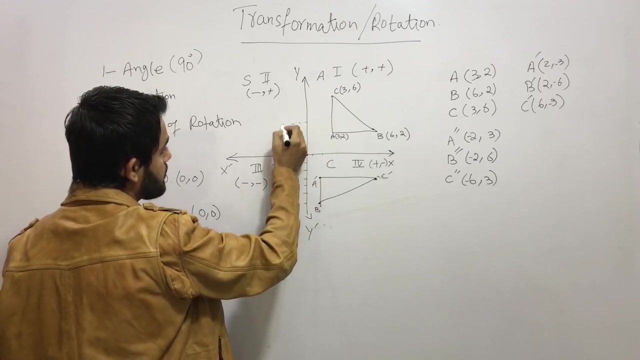 going to be minus, this is going to be minus and this is going to be minus as well. now take all these three points. so minus 2 comma 3, so this is x is minus 1. let's say this is going to be a minus 2 and for y it's 3. okay, so over here it's 2, so 3 should be a little up. so this is our first point. 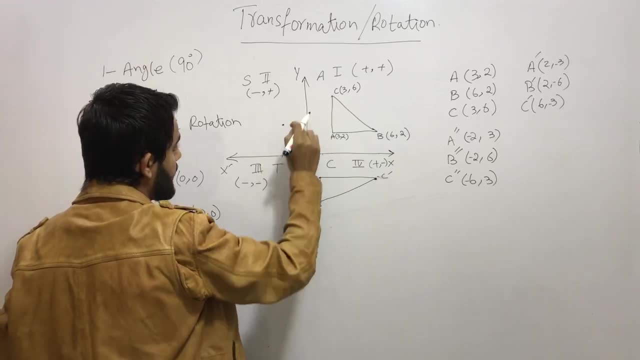 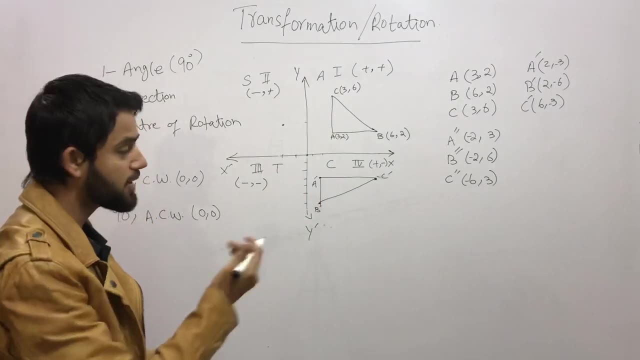 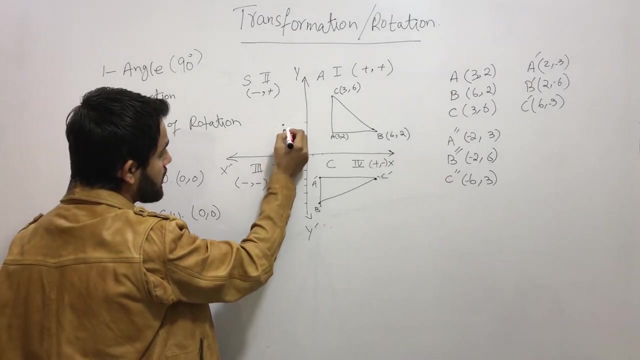 do not mind that i am taking random points and i'm trying my best to keep the same distance, but actually if somewhere it's not, you have to neglect it and try to learn the concept that i'm trying to convey basically. so the a point is minus 2 comma 3, so i'm going to write it as a double prime. 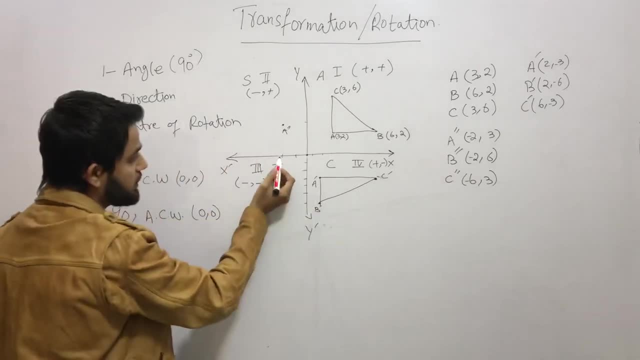 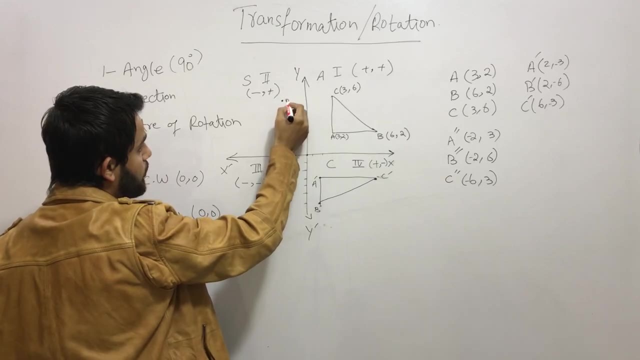 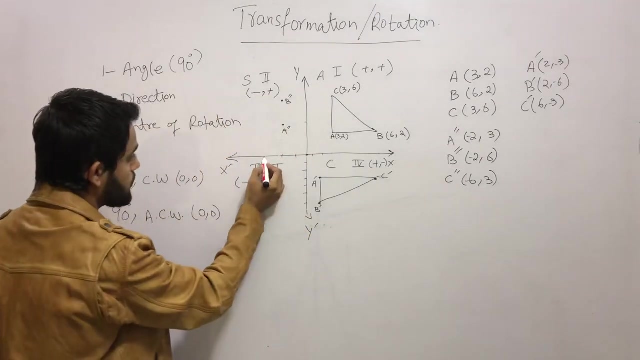 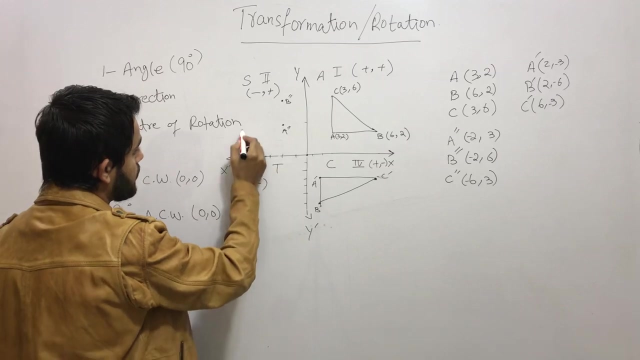 you Now. B double prime is minus 2, 6.. This is minus 2, 6. if it is 3 and 6 will be over here. So here we got B double prime and C double prime is basically minus 6, 3.. So minus 2, minus 3, here minus 4, minus 5 and minus 6, 3.. So 3 is here. 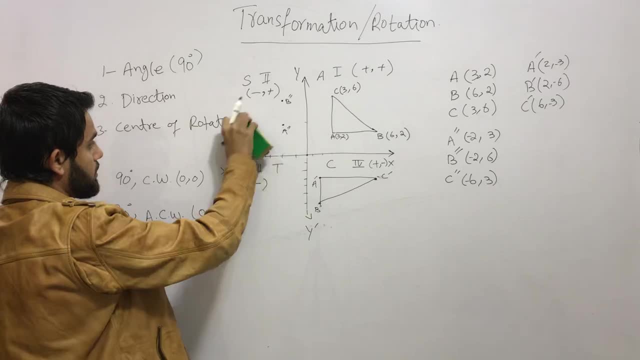 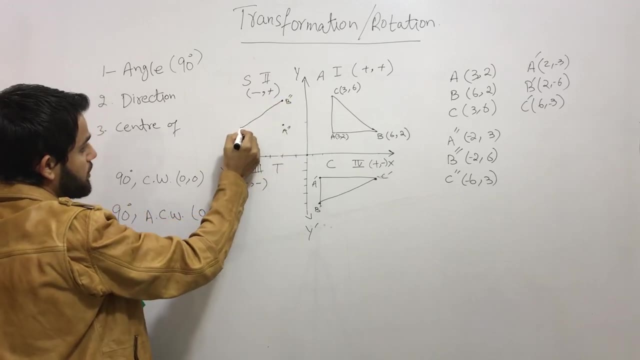 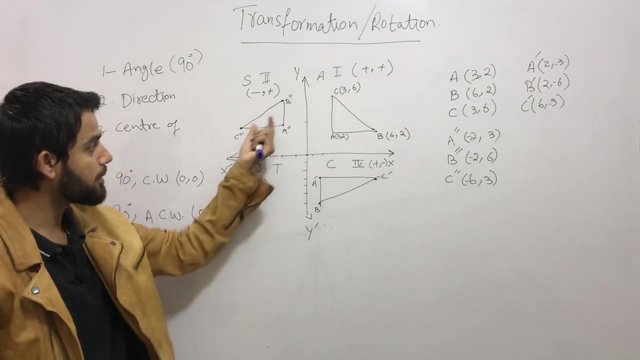 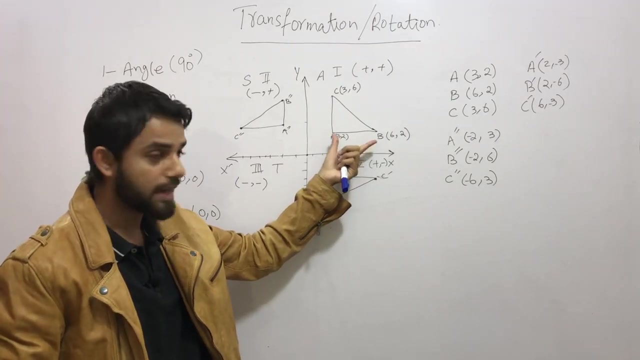 Let's remove this, and here we got C prime. Now join all these three points and here you go, And this is what we have got now: A double prime, B double prime and C double prime. So I have taken the same example and we have learned how to rotate triangle ABC 90 degree by keeping your center as an origin. 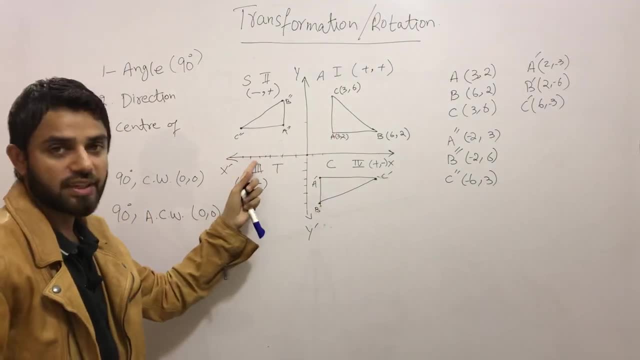 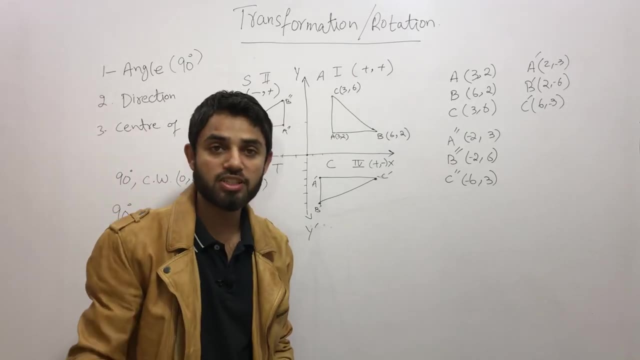 In clockwise direction and in anticlockwise direction. So this is what we have learned Now, what I am going to do now next. So in next we are going to learn about the rotation 180 degree, where we are going to keep the angle 180 degree. 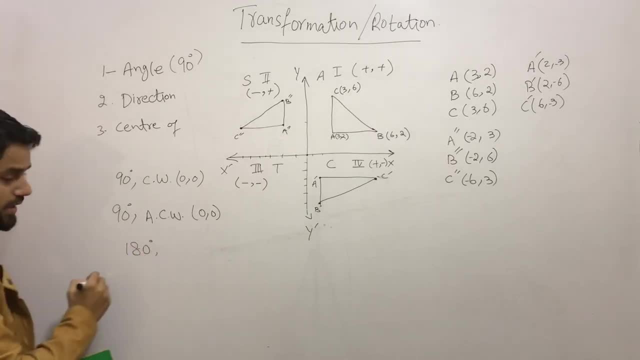 So now the same angle that we have got, 180 degree. I am going to keep the same triangle. Now the first we will be learning as clockwise. Now one more thing: Once you are having the angle, Basically 180 degree, In that you don't really need the direction, whether you are going as a clockwise direction or anticlockwise direction- 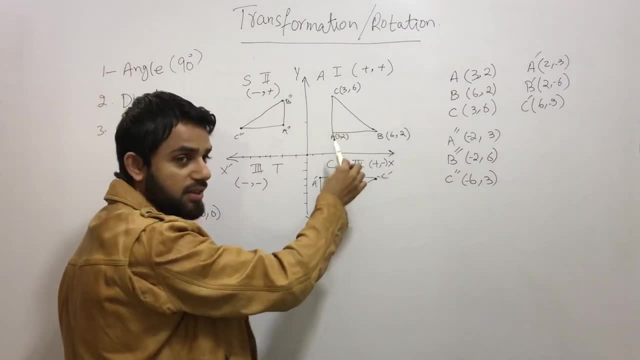 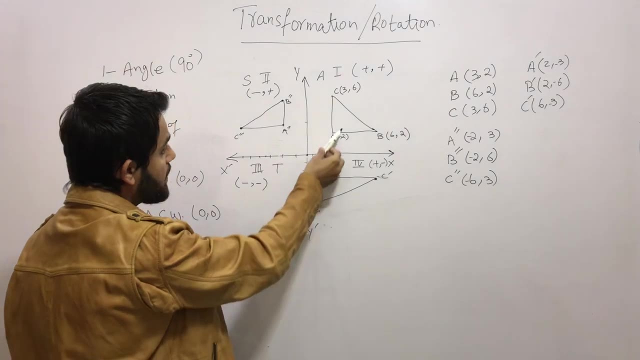 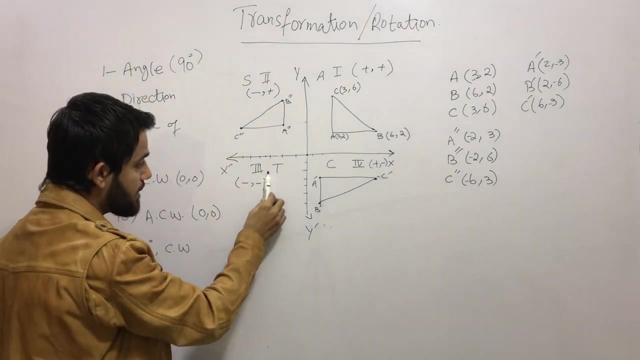 If you are having this triangle and you are trying to rotate it 180 degree- Let's say we are doing clockwise- You will be end up on this quadrant. So if you try to go anticlockwise by keeping this as a center, Now in anticlockwise direction again, you will end up on this quadrant as well. 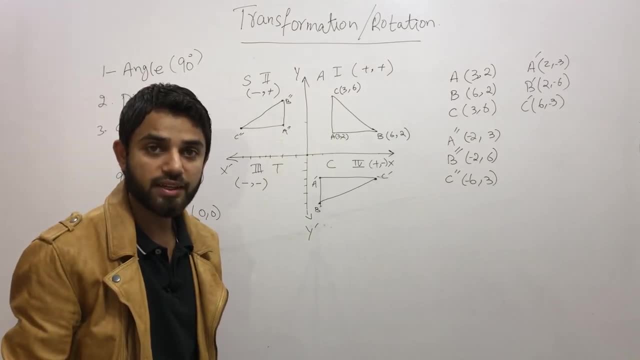 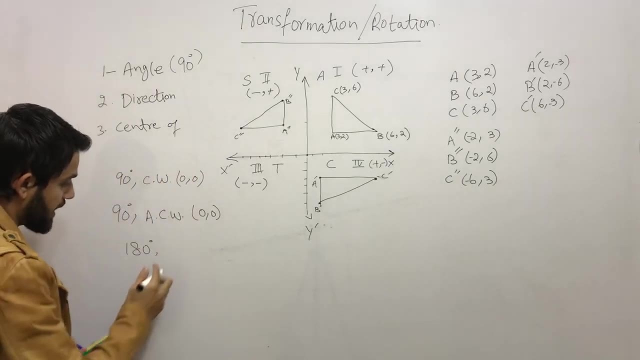 So for 180 degree Rotation or for 180 degree angle, You don't really need the direction from where you have to go. So we can neglect this part and I am writing 0 comma 0.. This is basically your center of point. 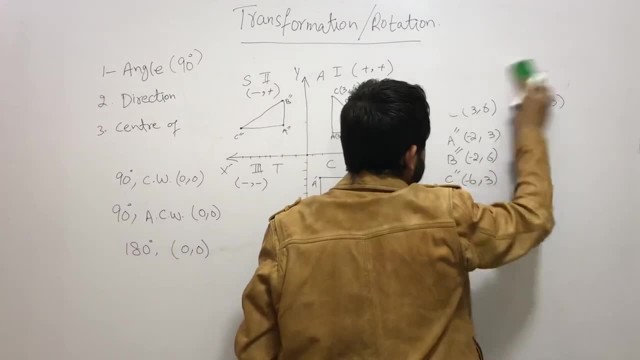 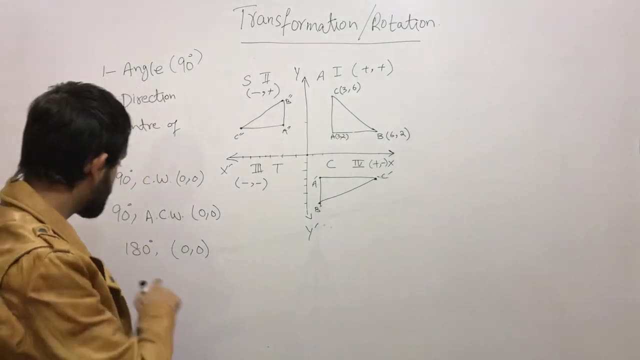 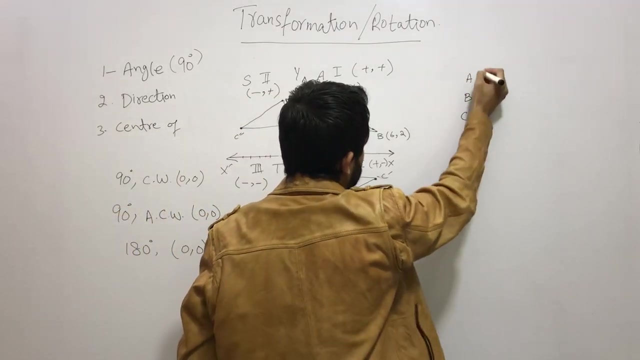 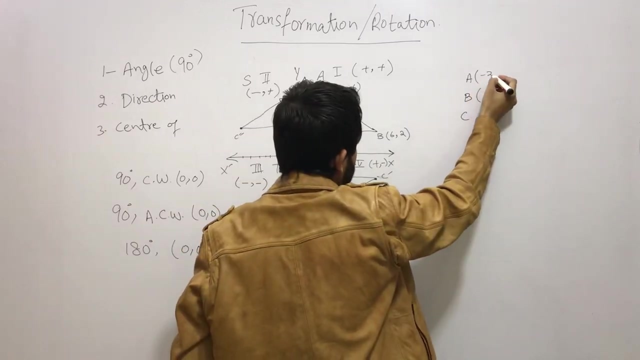 Okay, now I am going to take the same figure. This is ABC, and we are going to rotate it to 180 degree. Okay, so for 180 degree you have to do The opposite. So if your A is 3 comma 2. You are going to take the opposite of 3 will be minus 3.. 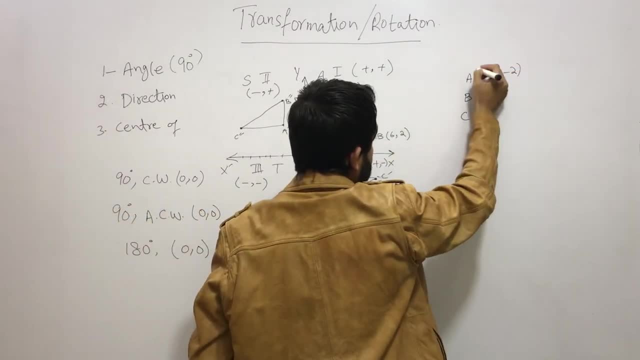 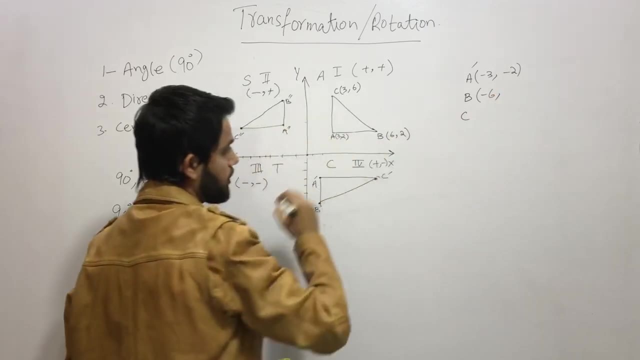 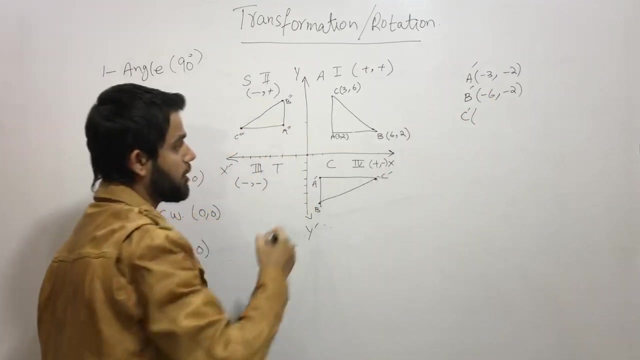 The opposite of 2 will be minus 2.. So this is going to be your A prime. Now for B prime. the opposite of 6 is obviously minus 6.. The opposite of 2 is going to be minus 2.. And the opposite of C for 3 is going to be minus 2.. 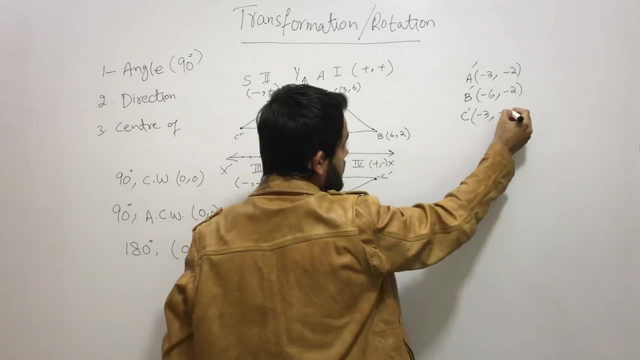 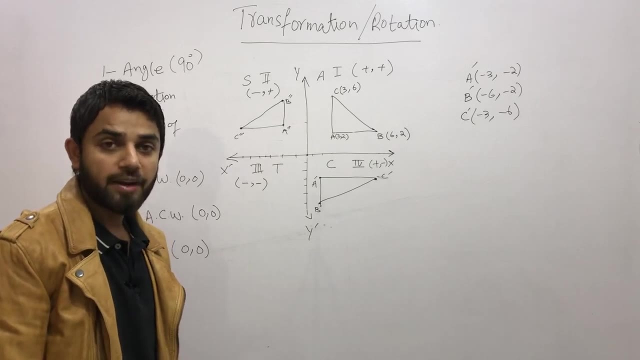 And for 6 it's going to be minus 6.. So now these are the three coordinates of the triangle ABC we have got by rotating in 180 degree angle, And the direction, we really don't care in that case, once we have an angle of 180 degree, 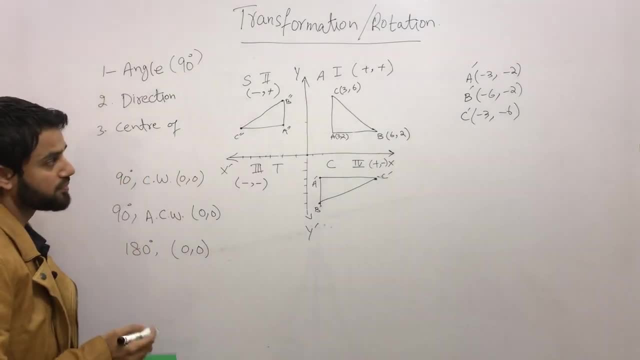 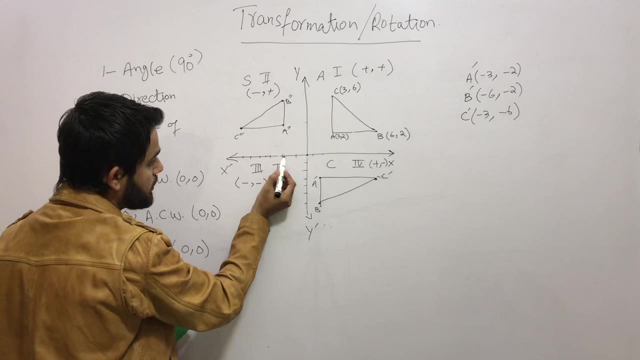 But the center of point. we do know that it's 0 comma 0.. Okay, so now the first point A is minus 3 comma minus 2.. So 1. 2. This minus 3 comma, minus 2.. Minus 1 minus 2.. 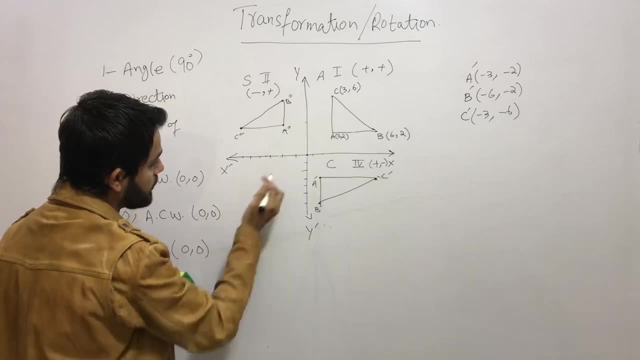 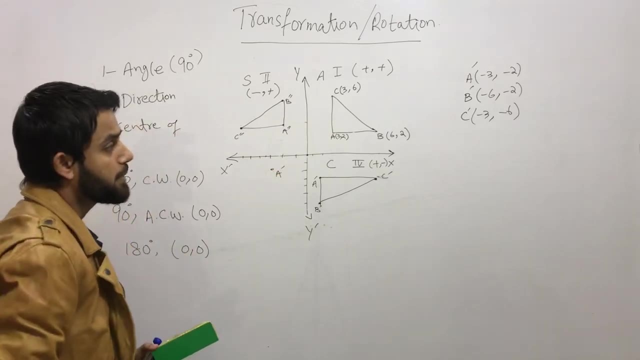 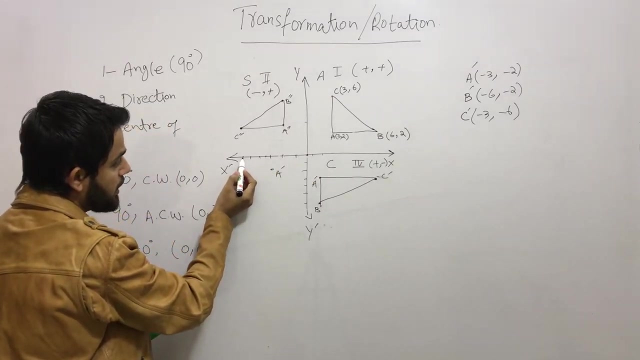 I am removing these. So 1., 2. Minus 3. 2.. So this is the point that we have got for A prime, For B prime minus 6 comma minus 2.. 1 minus 1 minus 2 minus 3 minus 4 minus 5 minus 6 comma minus 2.. 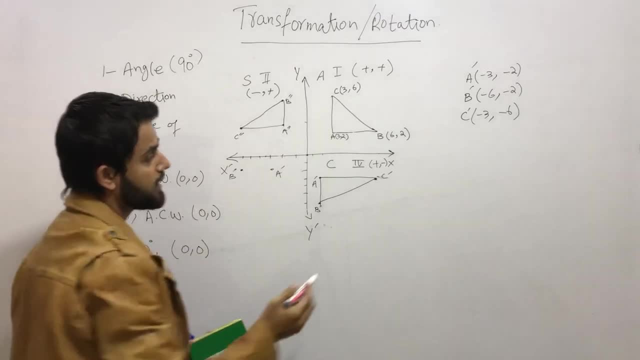 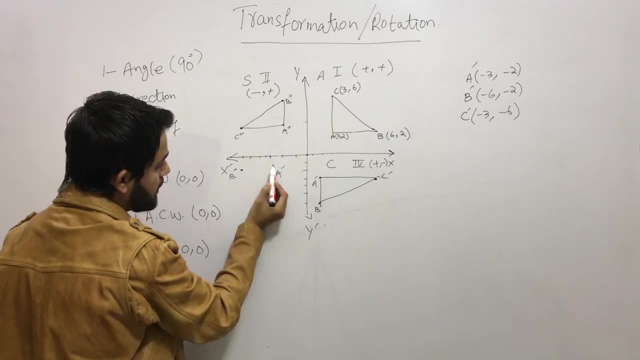 So this is the point that we have got B prime And then C prime. X is minus 3., 1., 2. Minus 3. And Y is minus 6.. So 1., 2., 3.. 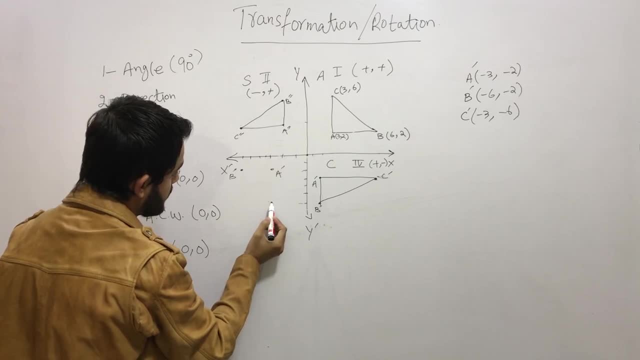 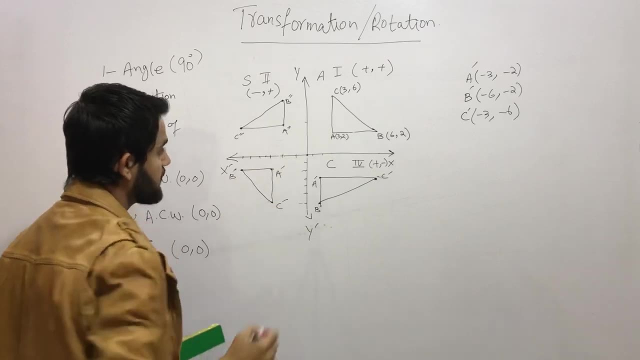 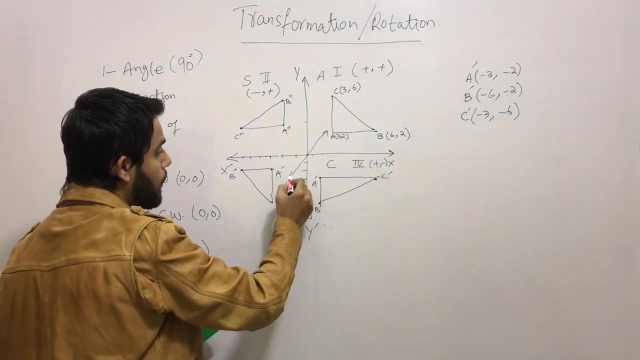 4. 5. 6.. So this is the point we have got for C prime. Okay, now join all these three points And this is what we have got once we rotate this original triangle ABP 180 degree, by keeping your center of point as 0 comma 0.. 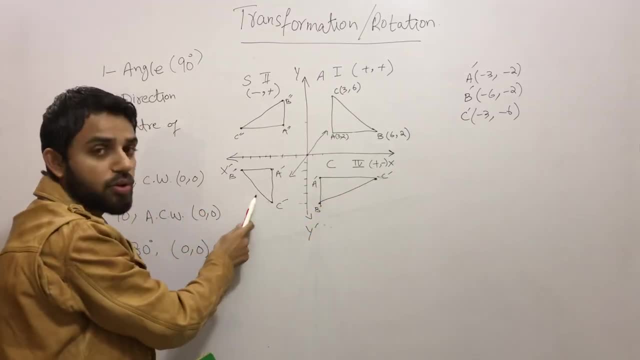 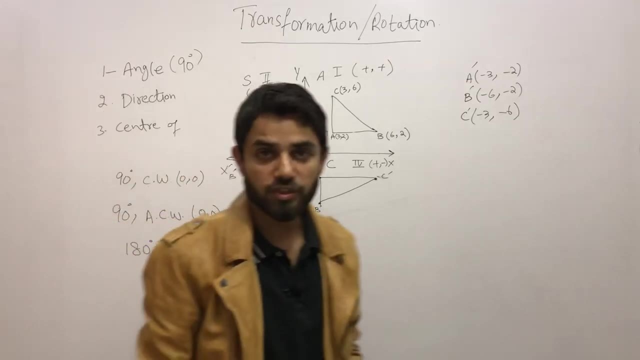 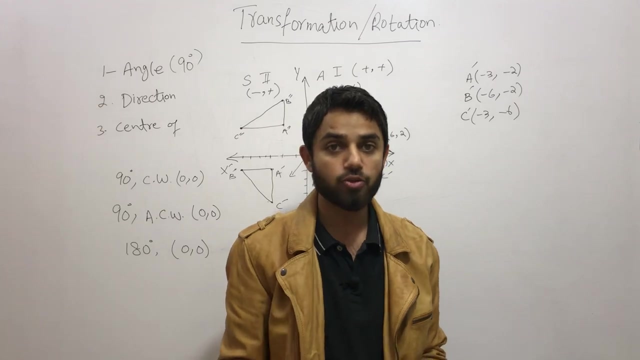 So if you, If, If you rotate the clockwise, you are going to end up in the same way, and by anticlockwise, you are going to end up in a same way as well. So I hope that this video was very helpful, helpful for you to understand the basic concept of rotation in transformation. that how do we have learned? 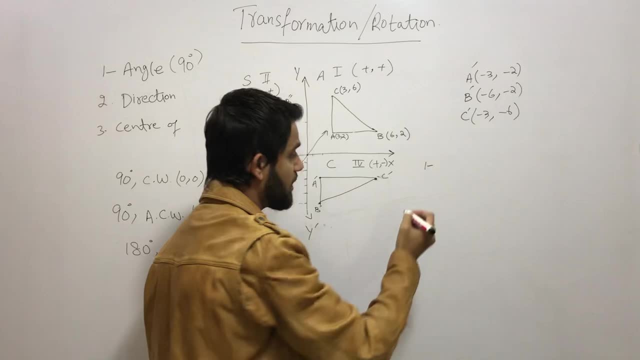 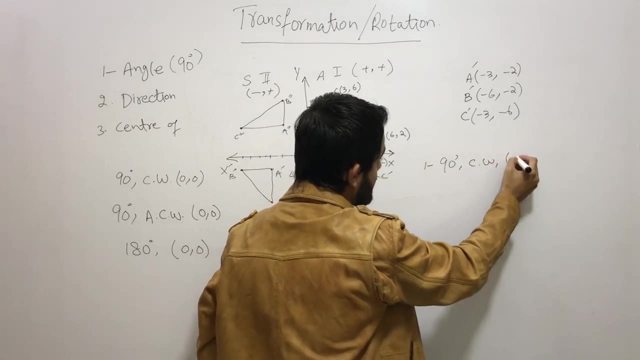 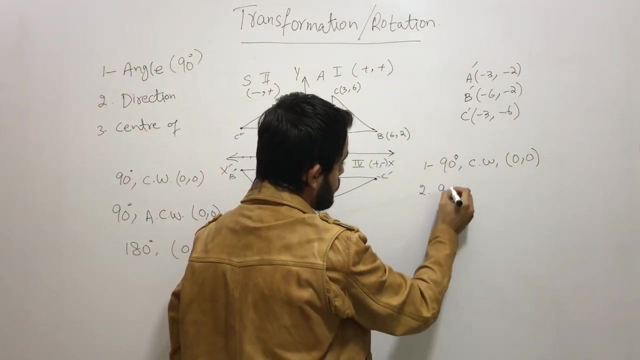 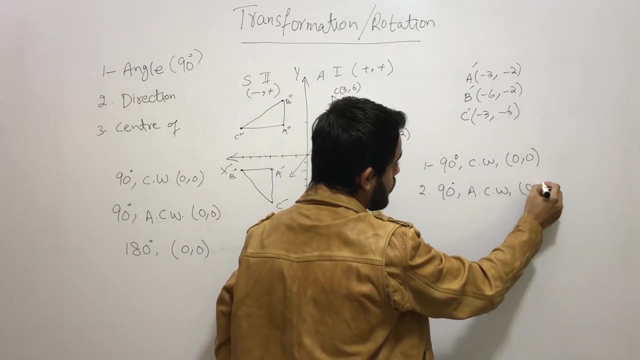 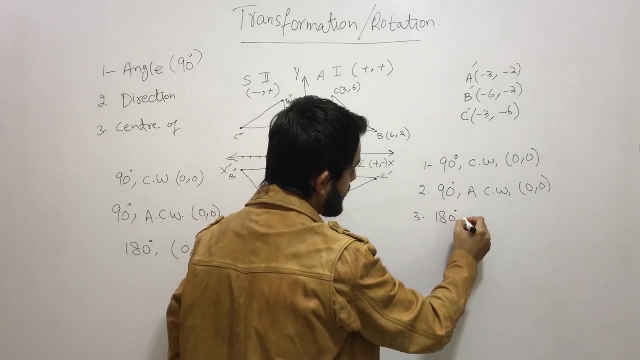 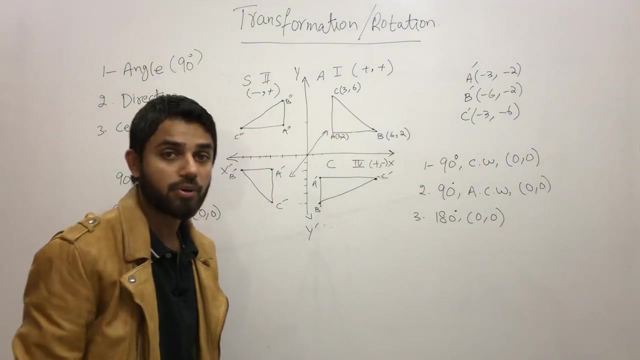 So what we have learned in today's video? we have learned the first thing that how to rotate an object 90 degree clockwise by keeping the center of point 0 comma 0. Then we have learned that how to rotate a figure 90 degree in anticlockwise direction by keeping 0 comma 0 as your center of origin. and then we have learned rotation with 180 degree angle- the direction I already told you we don't really care about that- by keeping 0 comma 0 as your center point. 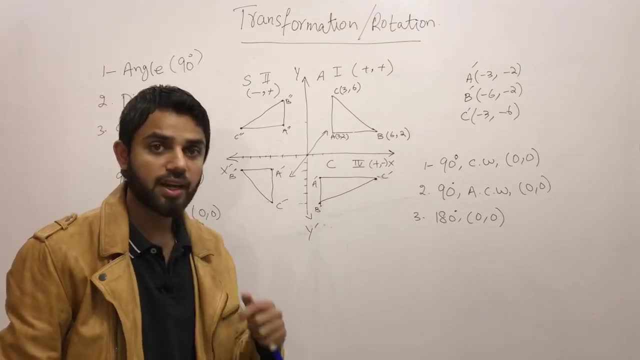 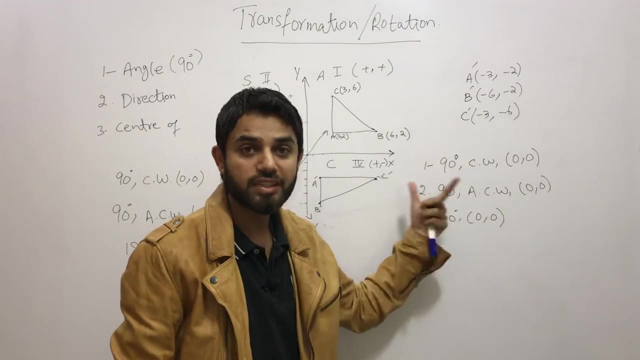 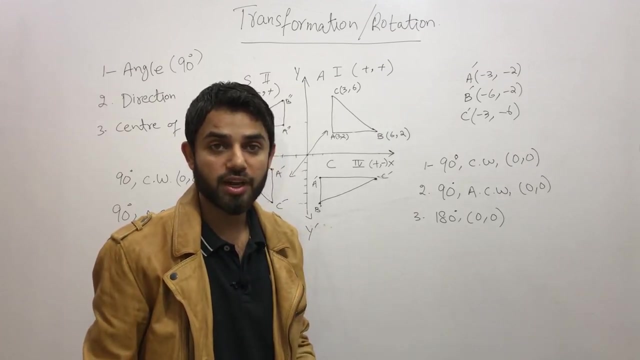 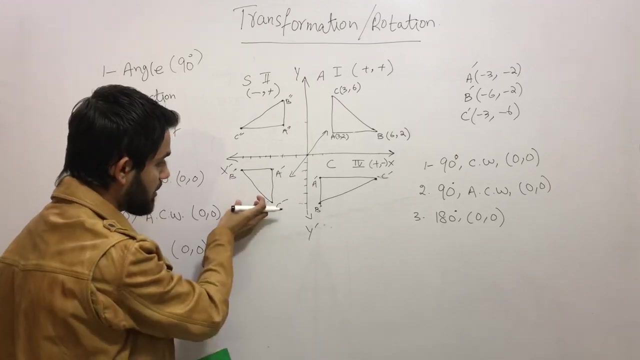 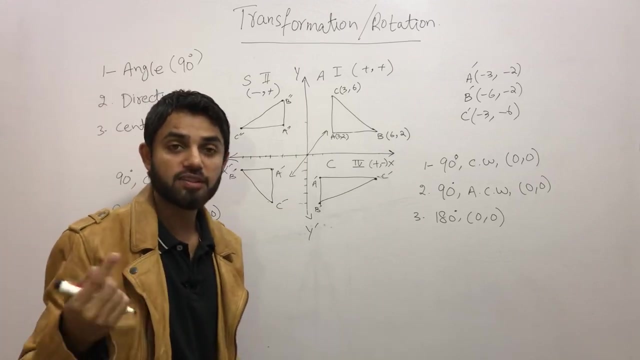 So there is one more thing that I would like to highlight over here That only the center of point 0 comma 0 or our region, that is not the only case. you can. you you will be having the point 2 comma 1 or sometime. if you are having or if you are appearing for your IGCSE or GCS exam, you might have been given the object and you might have been given the image and what you really need to identify that, which type of transformation it is. if you tell them that if it is rotation or reflection or translation, you will be given the image.